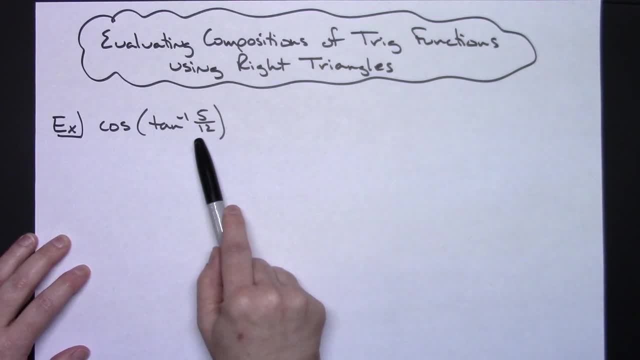 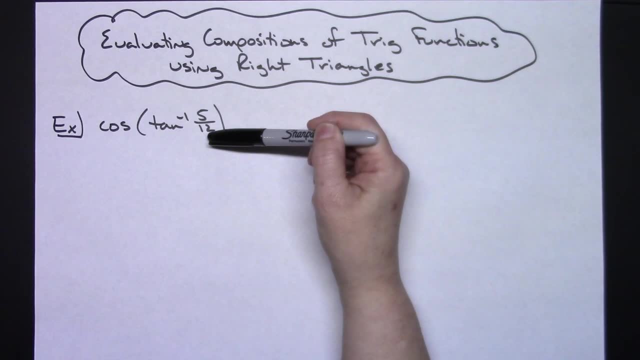 We're going to work on the inside part of the function first. We're going to recognize that this is 5 twelfths. So this is going to work. nice for us to be able to use that bowtie triangle And figure out which quadrant it should be in so that we can set up a right triangle. 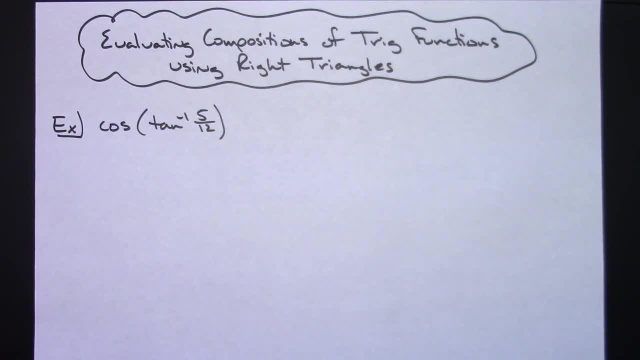 and then we'll be able to evaluate this outside function here. So to start with, we're going to, let say, theta equal to that inverse of tangent of 5 twelfths, Alright, which basically, if you remember, if you're trying to do the inverse, 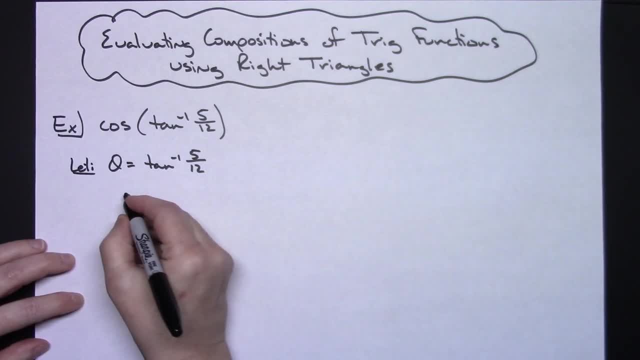 function. there you're trying to basically find the angle. So the tangent of theta is equal to 5 twelfths And I'm looking for that angle, Alright, so what I'm going to do is I'm going to want to draw my right triangle, So I have to figure out, okay, well, which one of those 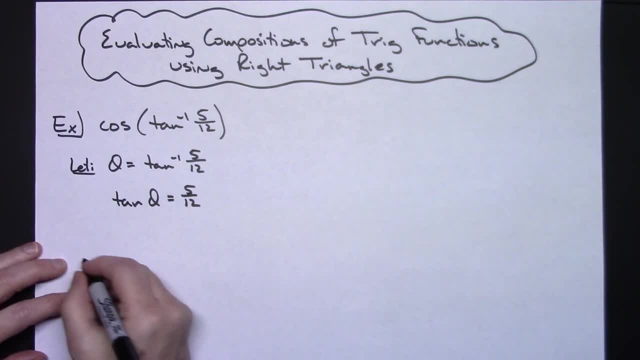 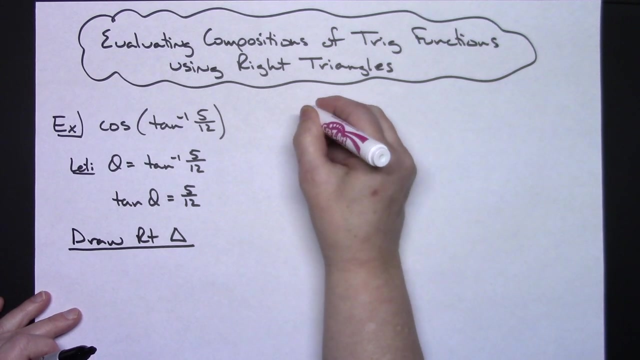 bowtie triangles, is it? Which quadrant does it lie in? So we're going to draw our right triangle, Alright, but let's write some stuff down over here to help with the placement of this, Okay, so So remember that your tangent restrictions are the open interval from negative pi over. 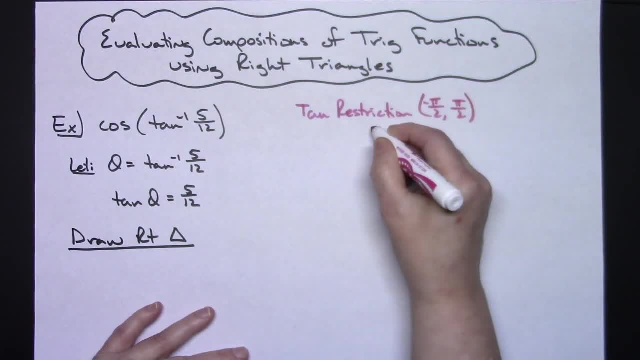 2 to pi over 2.. Alright, so real quick here. that means that my theta then would have to lie in here. Alright, so it can't be here and it can't be here. Alright, now, in my four quadrants here, go through and do the mnemonic that you have memorized, so that 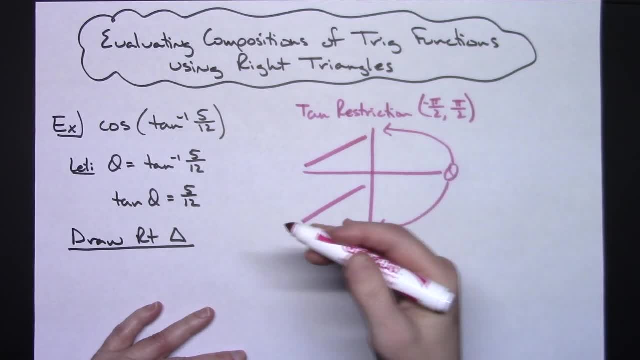 it tells you which trig functions are positive in which quadrant. So that would be all students take calculus. That's one mnemonic you can use which means all of the trig functions are positive in this quadrant. Sine and cosecant are positive in the second quadrant, Tangent. 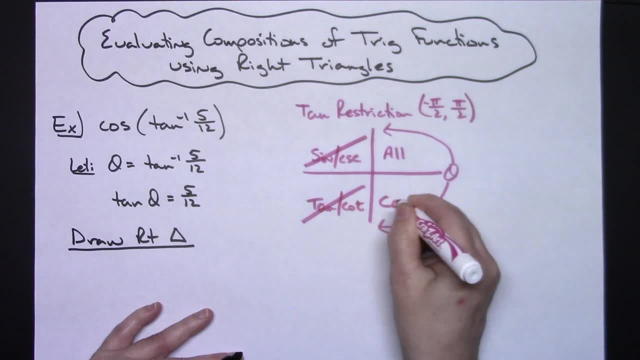 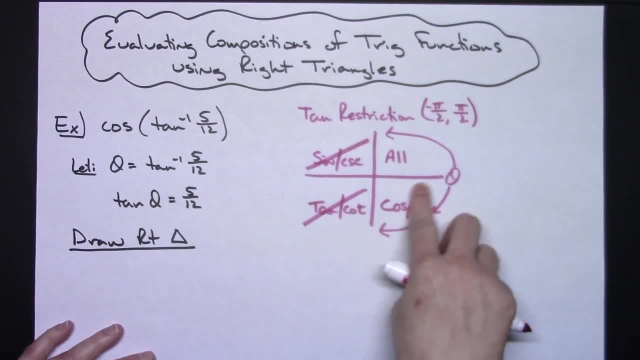 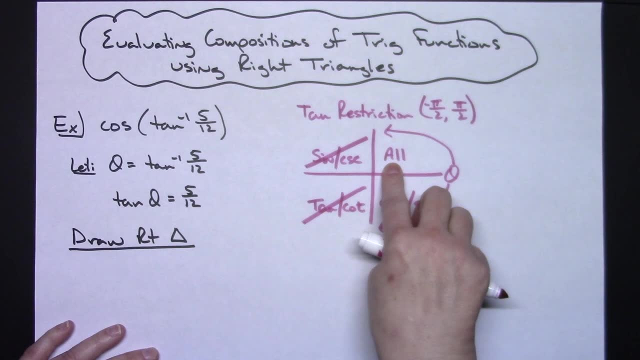 twelfths is positive, all right. well, down here in the fourth quadrant, tangent would have to be negative. up here in the first quadrant, tangent is going to have to be positive because all trig functions are positive here. so that tells me that when I draw my right triangle, the right triangle, part of the 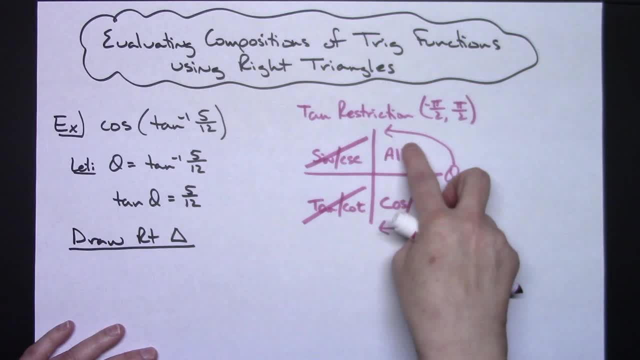 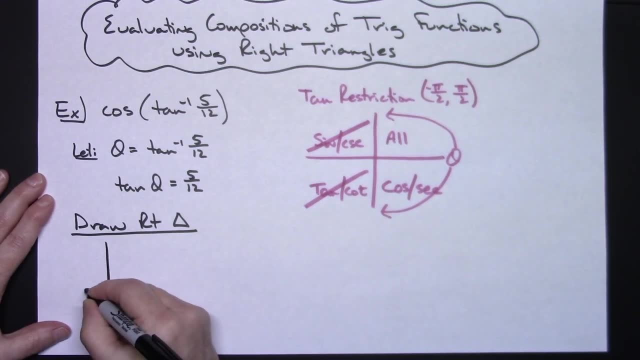 bowtie triangle that you are often taught in trig classes is going to have to be in that first quadrant there. all right, so I'm going to just real quickly sketch first quadrant here and I'm having that portion of the bowtie. all right, so my theta would be here, all right. tangent is opposite over adjacent. 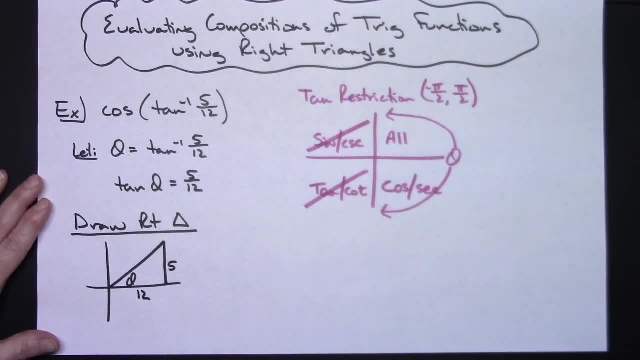 so that means this side has to be 5, this side has to be 12. all right, now that's a right triangle, so I can do Pythagorean theorem and I can do 5 squared plus 12 squared is going to be negative. so that's going to be negative, so I can do. 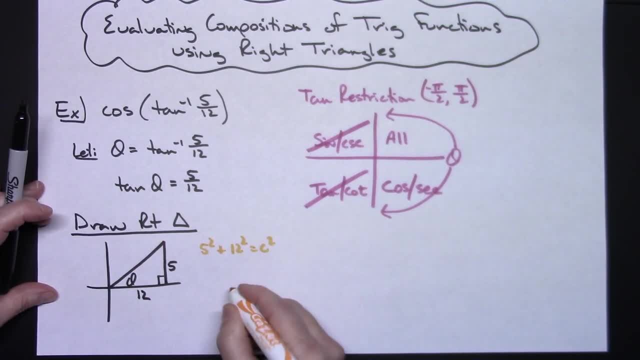 this and I'm giving a positive분 over here and I'll just start over. so this side is going to be negative and I'm going to guess this at that angle. so there is, this is the diagonal angle, and at thatятно angle. so here I'm, here I'm. 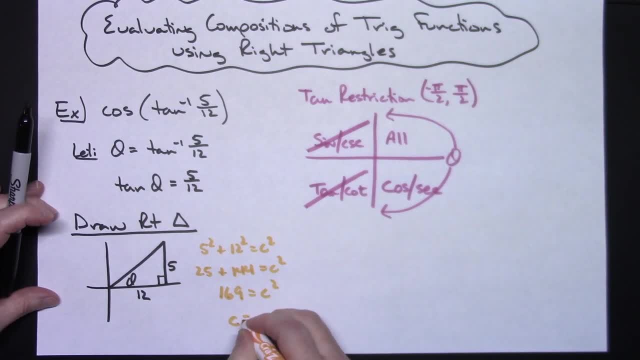 going to do this. I have from this coisas Arduino triangle, so I think that I'll bring this. here are all these areieth angles that I move. I'll go down and I'm going to smile in a way so that I know what they are. a plus π. 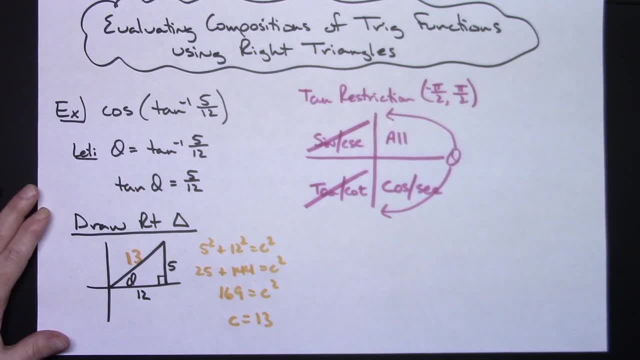 plus one terms as equals to. I think this is a great ι. I just figured out there could have some, or maybe something like this. so then, Okay, I've worked the inside out. This triangle represents the inside there. Now I just need to. I can use this triangle then and find the cosine of that theta. 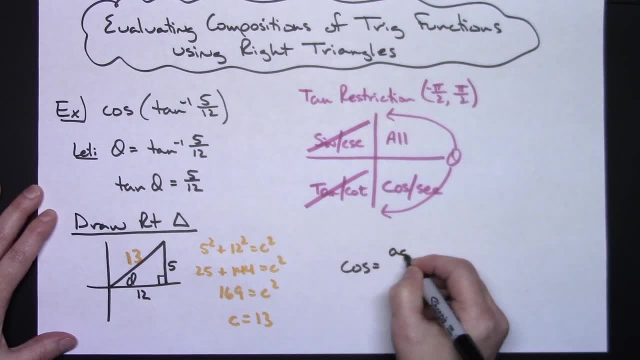 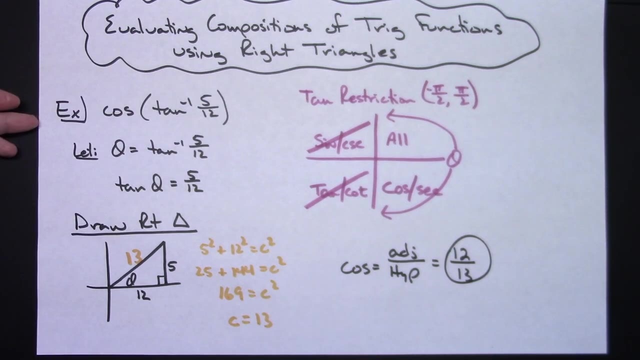 Cosine is, by definition, adjacent over hypotenuse, And so adjacent, which would be the 12,, and hypotenuse is the 13. So 12 over 13.. All right, so evaluating this composition here of trig functions. 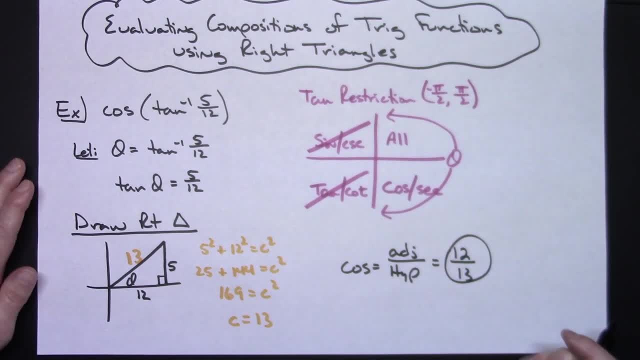 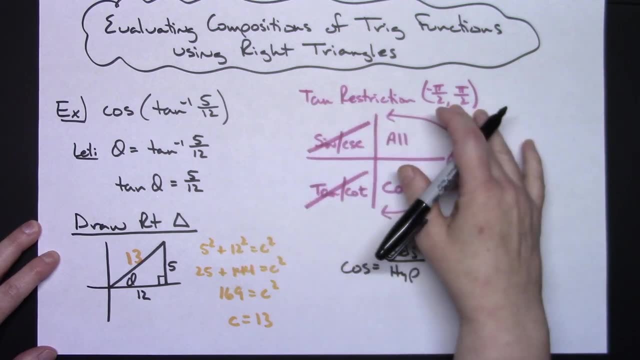 I get 12 over 13.. All right, so again, no calculator was needed. I'm using those bowtie triangles and keeping in mind what my restrictions are and where those trig functions are positive. All right, now let's do another one. 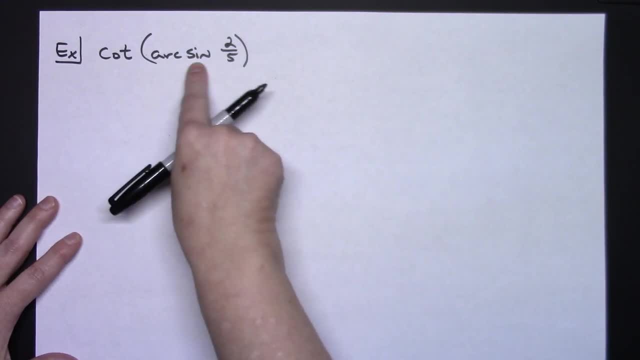 Okay, changing up the notation here just a little bit. All right, this really should be read the inverse sine of 2 fifths, but a lot of people say arc sine of 2 fifths. right there, All right, so we're going to work this one out. 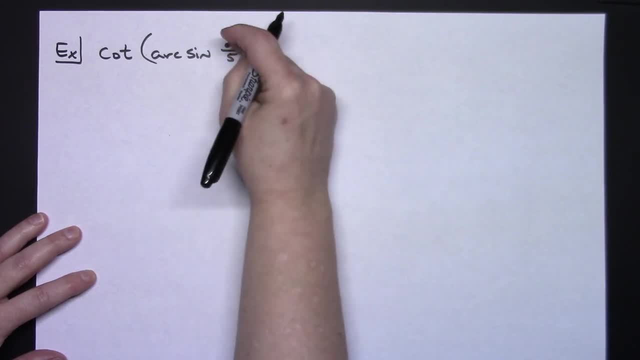 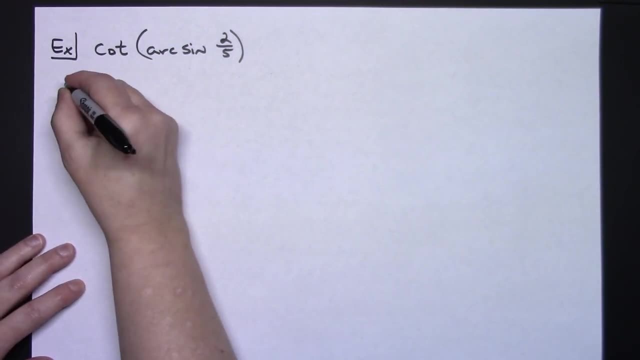 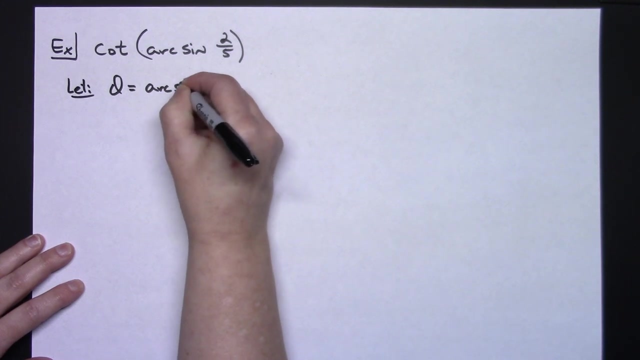 We're going to do the exact same thing. We'll start on that inside part. The fact that this is a fraction is a good indication to tell me that I'm going to be able to use these right triangles to evaluate this. So I'm going to let theta equal the inverse of sine of 2 fifths. 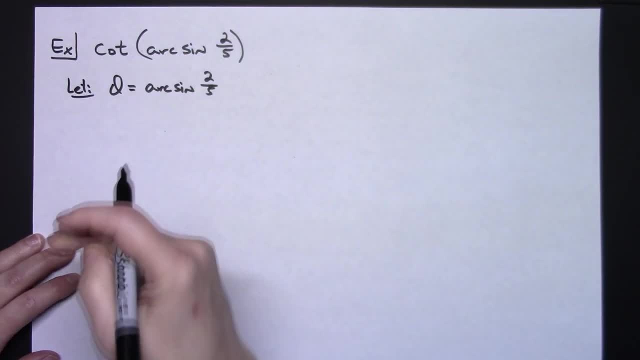 Again- oops, that didn't look like 2 fifths. Again, that should tell you that you're hunting for the angle all right, whose sine is 2 fifths. So I'm trying to go backwards. I'm trying to go backwards and find that angle. 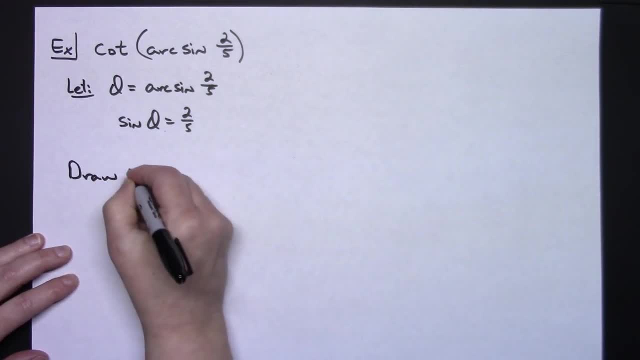 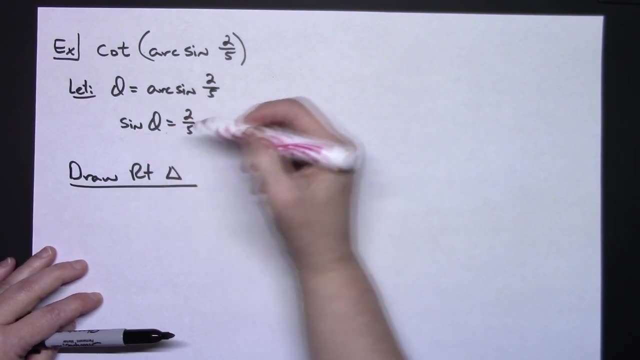 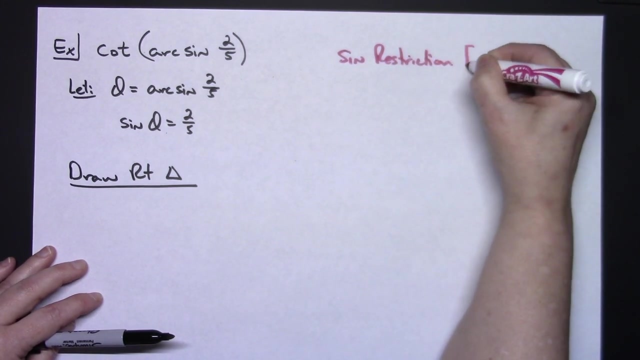 All right. so I need to have a right triangle. So I'm going to draw my right triangle, All right, but let's do some thinking here. On this one, I'm going to have to look at my sine restrictions. My sine restrictions- all right, are going to be the closed interval. 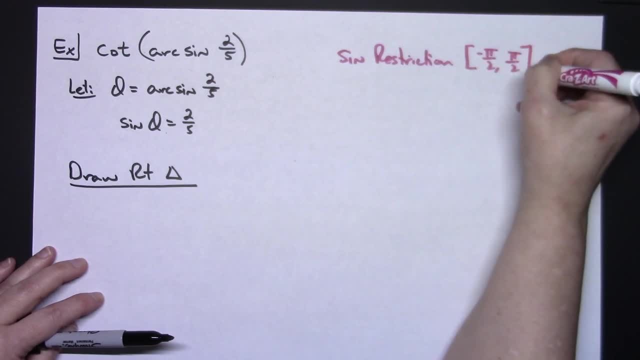 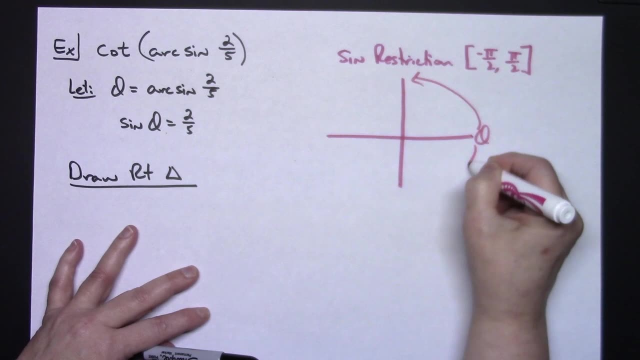 from negative pi over 2 to pi over 2.. All right. so if I draw a nice little coordinate plane here again, that means theta is going to fall. It's going to fall in these two quadrants. so not this one and not this one, all right. 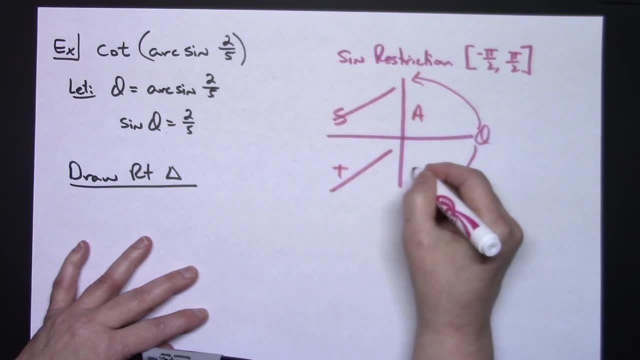 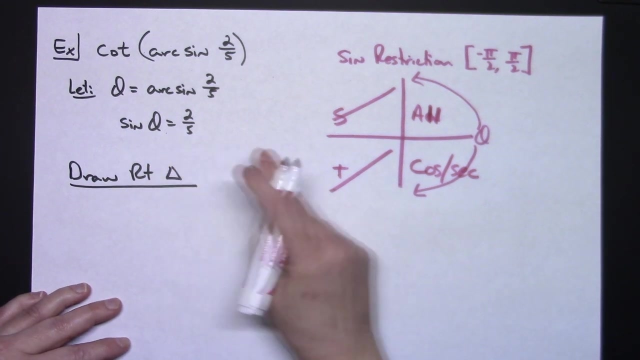 doing the. all students take calculus, All right. that means all of the trig functions are positive here. Cosine and secant are positive here, All right. so I have sine and I have a positive 2 fifths, All right. well, in the fourth quadrant there. 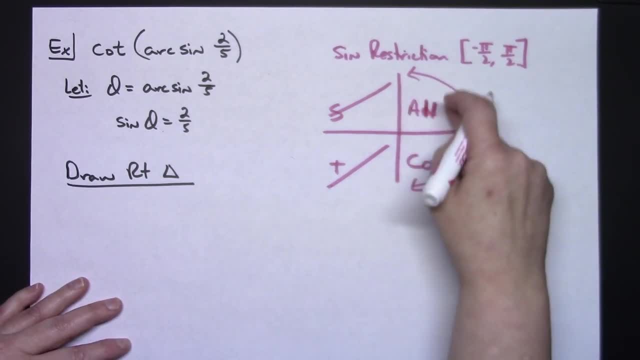 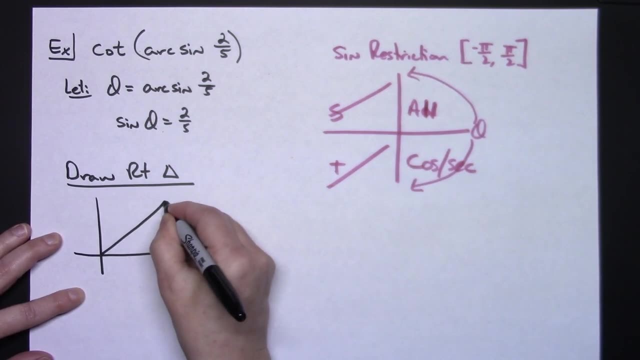 sine is going to be negative, so it can't be in the fourth one. Again, this example is ending up being in the first quadrant. So when I draw my right triangle, I'm going to draw it in the first quadrant. My theta is going to go here: 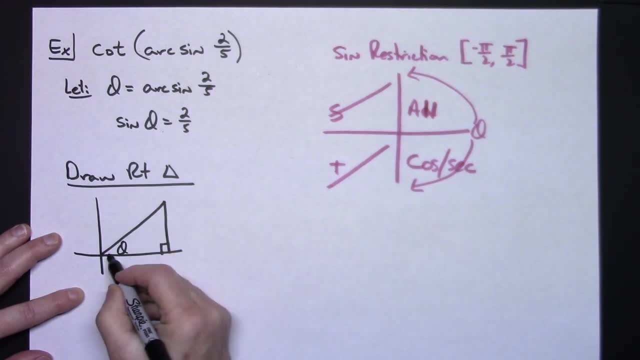 Definition of sine is opposite over hypotenuse. so opposite puts that side here, Hypotenuse puts the 5 there Again, Pythagorean theorem there to find that missing side. All right, so it really wouldn't make any difference here.